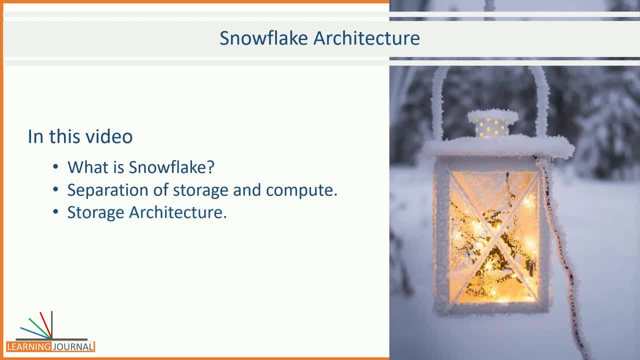 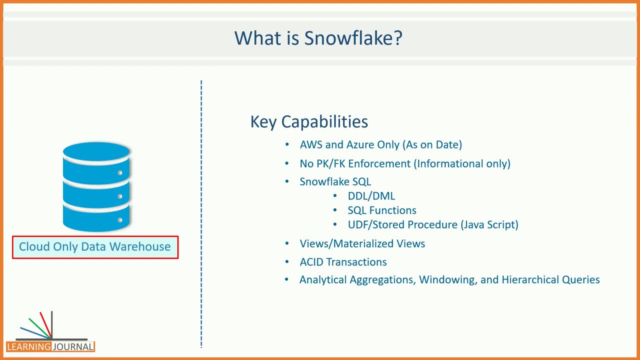 So make sure you watch it to the end. Let's start. What is Snowflake? Snowflake is a data warehouse that runs entirely on cloud infrastructure, And it cannot be run on a private cloud or on a hosted infrastructure. It is primarily available on the cloud. 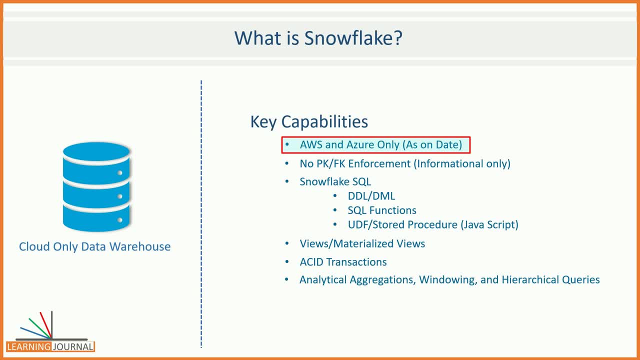 It is available on AWS and also available on Azure Cloud Platform. You should always remember that Snowflake is not a relational database, So it doesn't enforce primary key and foreign key constraints, But it offers Snowflake SQL commands like DDL, DML and SQL functions. 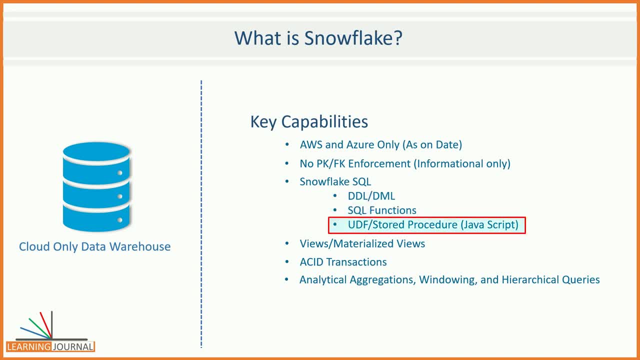 It also allows you to create user-defined functions and stored procedures using JavaScript. In this video, I am going to talk about how Snowflake works. Interesting right. The Snowflake SQL is rich enough to meet most of the data warehousing requirements. 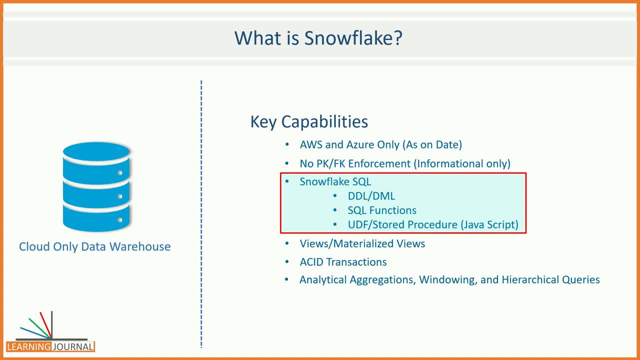 It supports select statements, joins sub-queries, insert, update, delete, merge statements, views, materialized views and AC transactions. It also supports common analytical aggregations such as cube, rollup, grouping, sets, windowing functions. 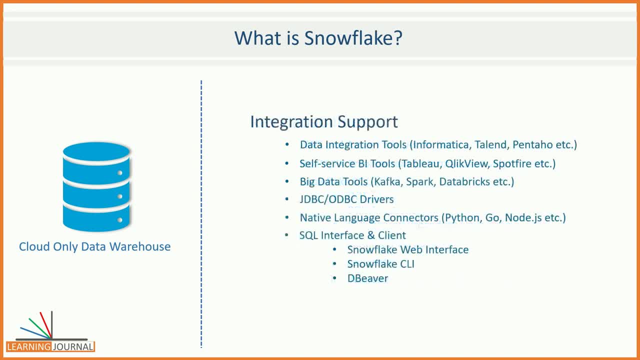 Like any typical data warehouse, it allows connection from most of the popular data integration tools, self-service BI tools and visualization tools such as IBM, Data Stage, Informatica, Talent, Pentaho, Power BI, Tableau, Clickview, Spotfire, Apache, Kafka, Apache, Spark and. 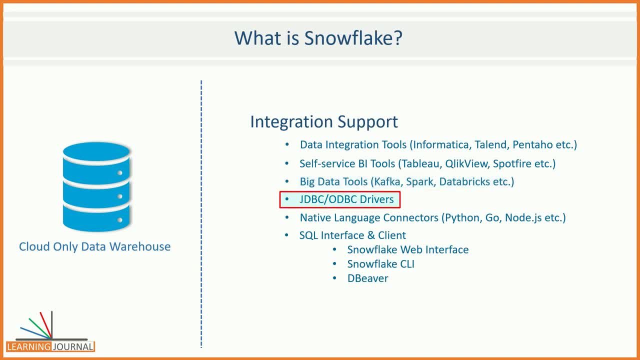 Databricks. If this is not enough, you can use JDBC, ODBC or any of these tools. You can also use the Cloud Platform. You can also use the Cloud Platform. You can also use JDBC drivers to connect from your application. 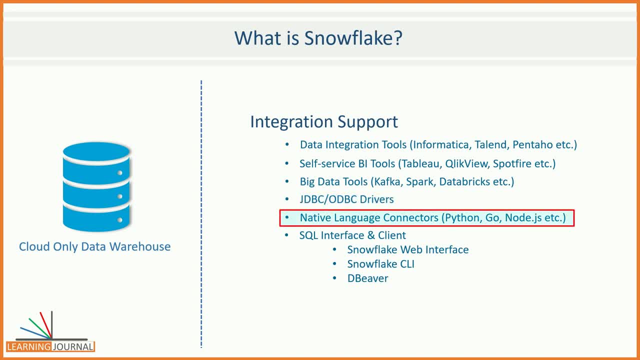 You will be amazed to know that it also offers native connectors for languages like Python, Golang and Nodejs. For ad hoc querying, you can use a Snowflake web interface which offers almost every feature that you would expect from a SQL worksheet or a database IDE. 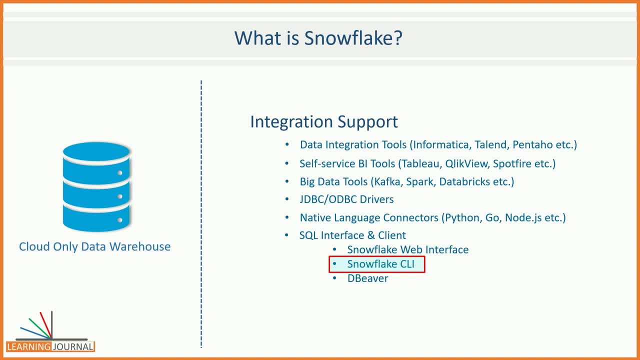 Alternatively, you can install Snowflake's CLI on your local machine or connect using DBAwer- Again, impressive right, But I am not yet, Because all this is anyway offered by almost every data warehouse system. What makes Snowflake different? 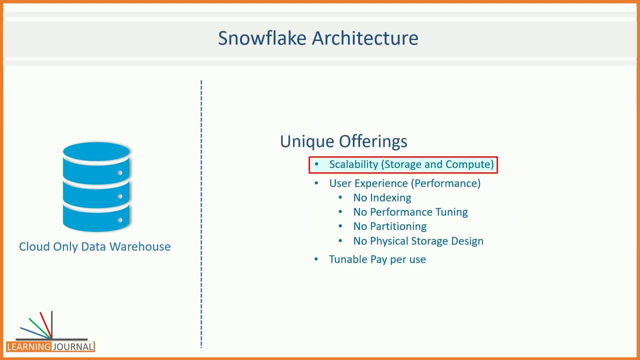 Well, it is the Snowflake architecture. The Snowflake system is designed in a way to scale and perform without any indexing, tuning, partitioning and physical storage design considerations, So you do not have multiple knobs to tune the database performance. 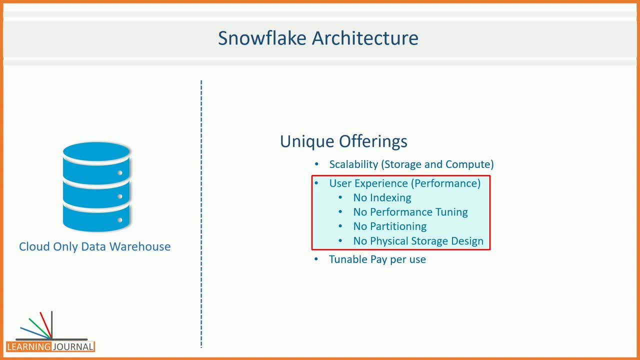 It just works- at least what the vendor claims- But you have few of the knobs to tune your cost and optimize your pay-per-use bills. Sounds interesting? Yes, it is. Let's try to understand how this fantastic data warehouse system architecture is designed to. 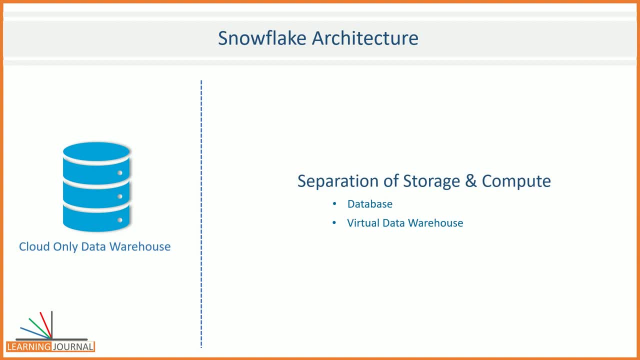 achieve all that. The first great thing that the Snowflake does is a real separation of storage and compute resources. In Snowflake you will have a notion of two things: Database and virtual warehouse. The database is the storage layer. It allows you to define a database, a bunch of schemas, and then add tables to the schema. 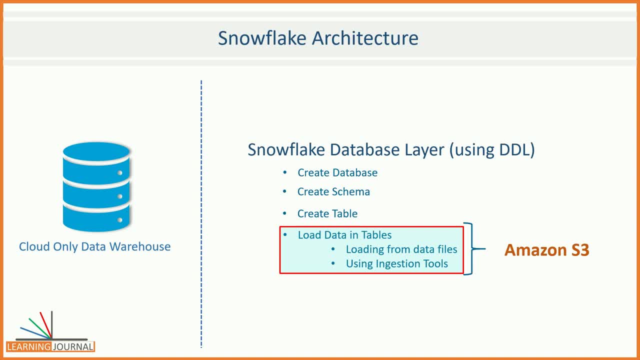 Once you have tables, you can start loading data into those tables. This is the typical structure that we follow in any data warehouse, right? But there is one thing which is unique in Snowflake: The data in the tables are stored in Amazon S3.. 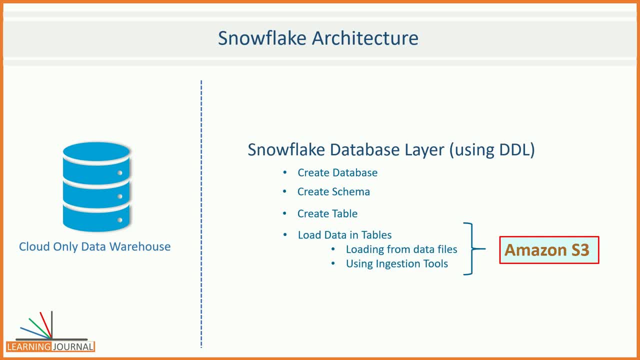 And it consumes storage-only cost. There is no compute cost attached to the database unless you are executing DDL or DML queries. What it means, You will pay for the compute cost. You will pay for the database. You will pay for the database. 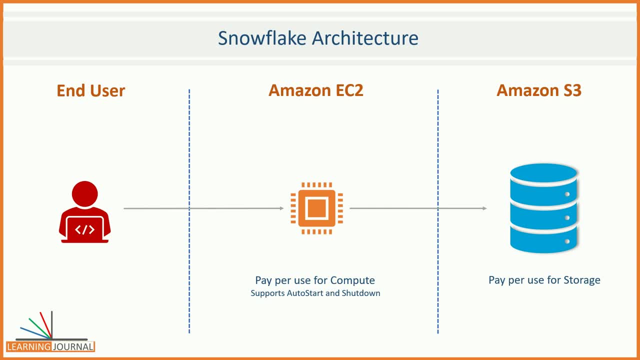 You will pay for the compute cost while you are running DDL statements to create a database, a schema table or other structural objects. If all these activities take 30 minutes, you will pay for 30 minutes of compute cost. Once your table structure is in place, you would want to load some data into your tables. 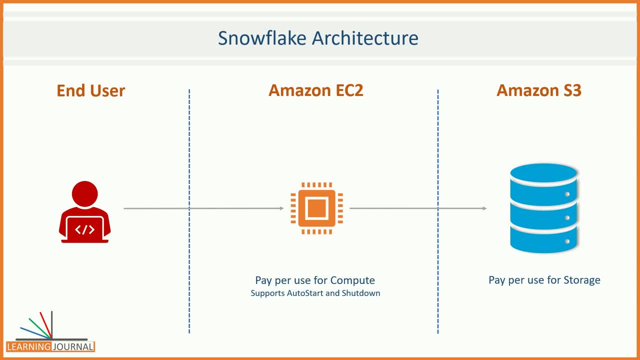 If your data load job is running for an hour in a day, you pay for the compute cost for an hour. Most of the time, you will be paying only for the storage cost. Similarly, if you are running queries for three hours a day, you will be paying to compute. 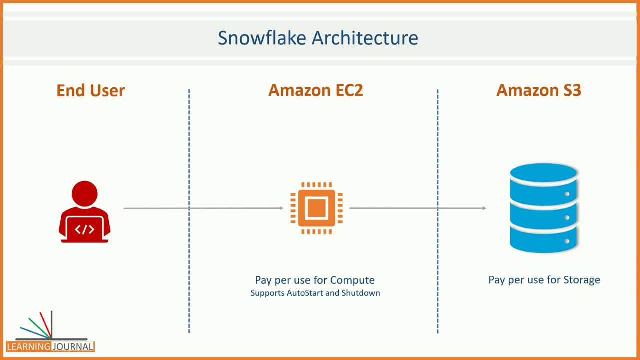 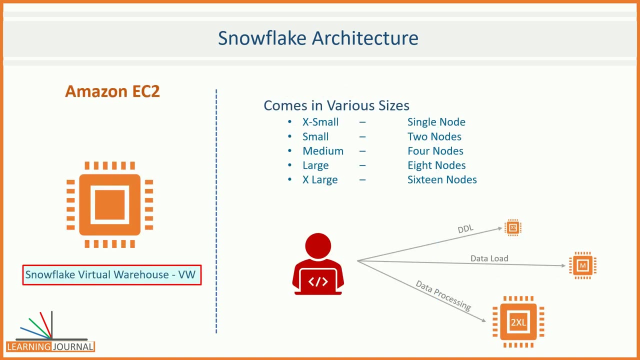 cost for those many hours. That's how it works at a high level. The next part of the Snowflake is the virtual warehouse, which is nothing but a compute cluster. They are named after virtual machines, but instead of machines, Snowflake termed them. 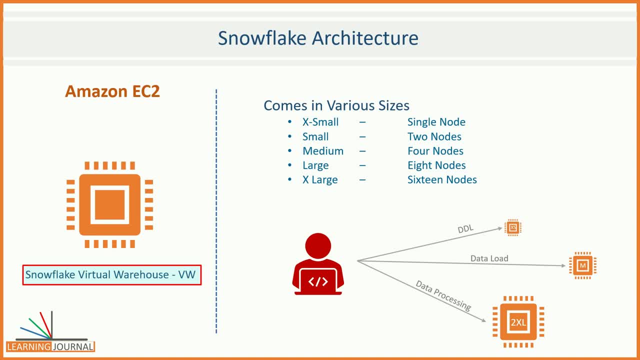 as virtual machines. In short, we call them VW instead of VM. You can create VW of various sizes, depending upon your requirement. It could be a single-node VW or it could be a multi-node VW, such as 2 nodes, 4 nodes. 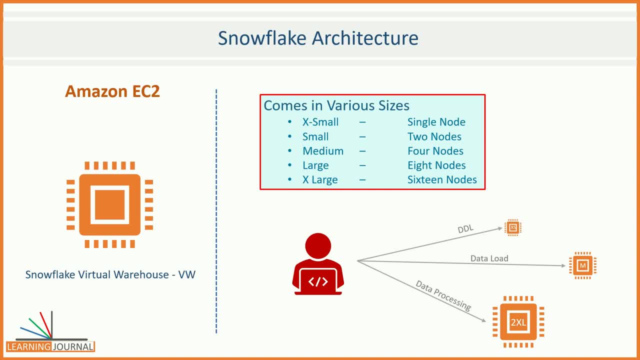 8 nodes, 16 nodes and so on. These nodes are nothing but Amazon EC2 instances, but they are internal to VW and you don't directly interact with them. Creating a VM does not have any cost associated with it. It is just a metadata creation. 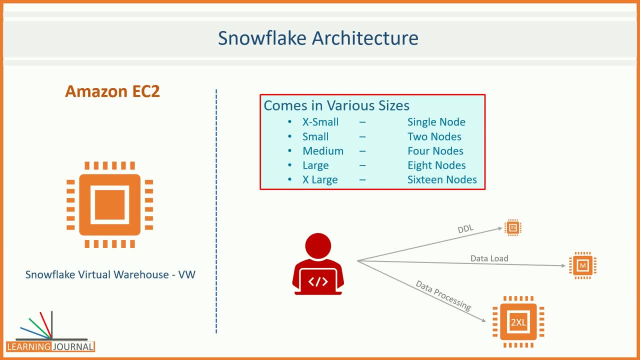 And you can have more than one VW configuration. For example, you might want to create a single-node VW for executing DDLs or performing some other low-resource-consuming activities. At the same time, you can also define a four-node VW which you want to use only for the data. 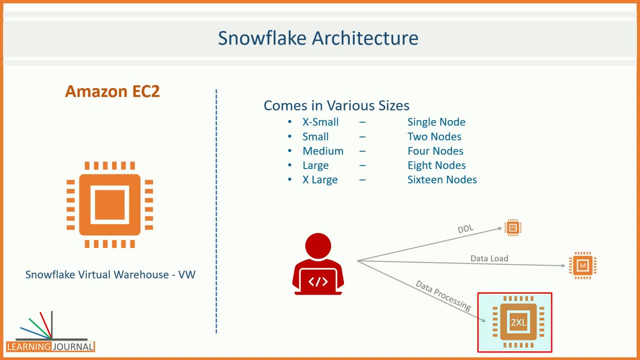 loading activity And you can create one more, a 32-node VW, which you wish to apply for a high-performing computation job that triggers every hour and completes in less than five minutes. The point is straightforward: You create your compute resource definition and start it only when you want to do some. 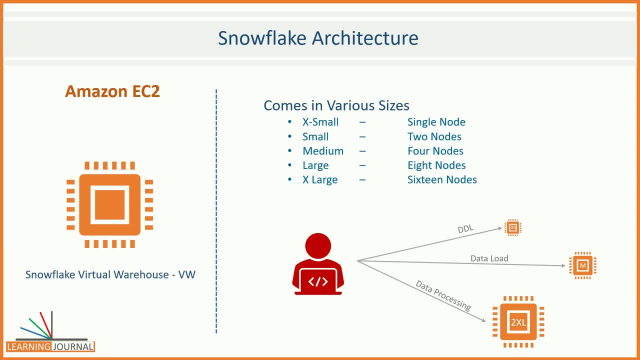 computation and shut it down when the computation activity is over. In this way, you pay the compute cost, And the best part is that you know which job is costing you how much money. Right, A job that runs for five minutes on a 32-node VW and triggers 24 times a day is charging. 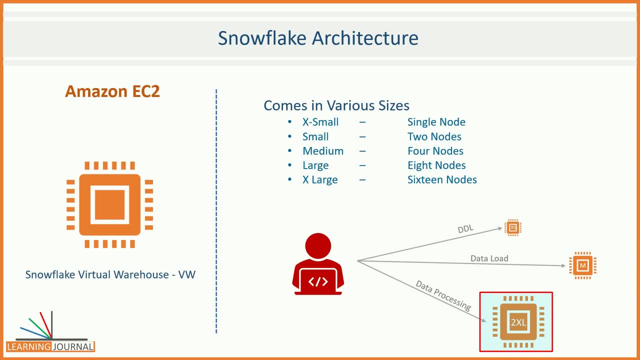 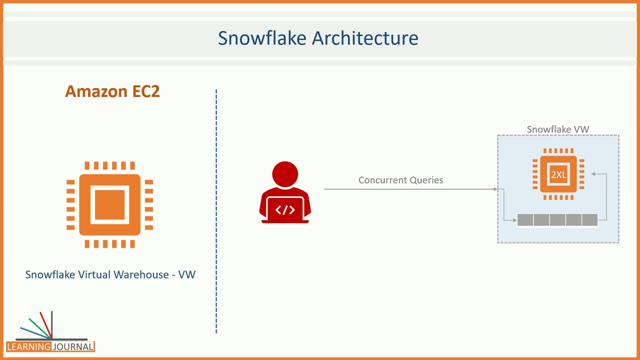 you for two hours of a 32-node VW Right, And that's valuable information for the business, isn't it? You can also use the same VW to execute multiple concurrent tasks- Right queries. In that case, as the queries are submitted to the same VW, the warehouse allocates resources. 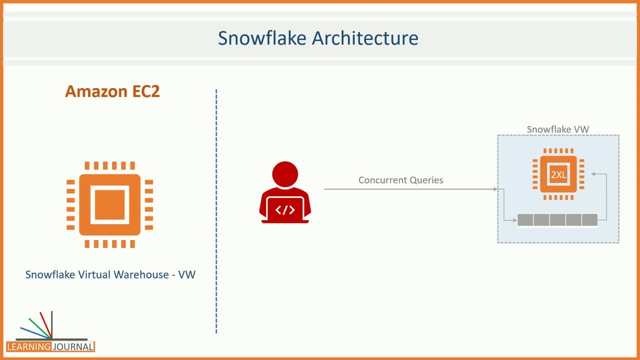 to each query and begins running them. If sufficient resources are not available to execute all the queries, additional queries will be queued until the necessary resources become available. So you have all the flexibility to plan the compute workload and reuse your VWs. The notion of VW doesn't stop there. Snowflake also offers a unique idea of multi-cluster VW. 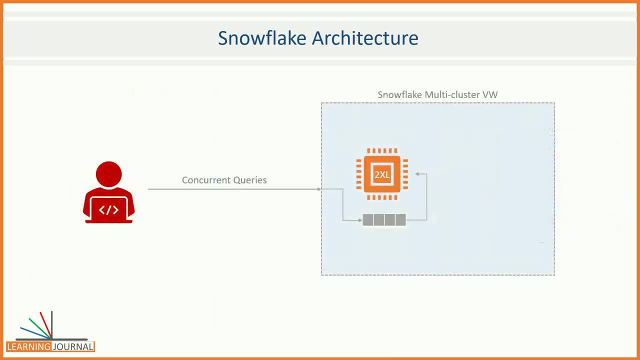 for auto-scaling. For example, you created a multi-cluster VW and started a query on the VW. Snowflake would start your query normally in the same VW. However, if you start submitting more and more queries on the same warehouse, at some point they will consume all the resources. 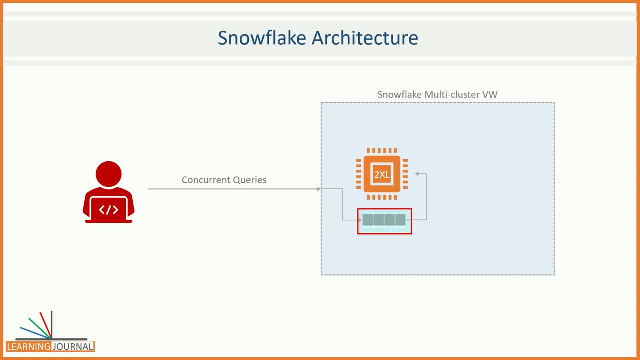 that are available to execute all the queries. So you have all the flexibility to plan the VWs and additional queries will be queued until existing ones are complete. But you created a multi-cluster warehouse. A multi-cluster warehouse will detect this scenario and automatically. 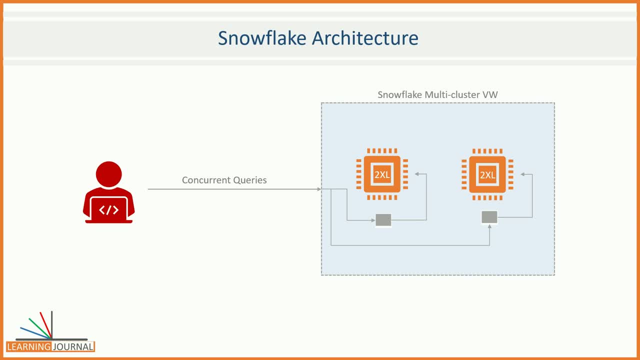 launch a new warehouse to execute the queued SQL. The point is straightforward: Snowflake allows you to configure automatic scale-up by starting additional VWs and scale-down by shutting down the VWs depending upon the workload. This feature is powerful if you have strict performance SLEs. Great, So you can draw a high-level architecture diagram using the. 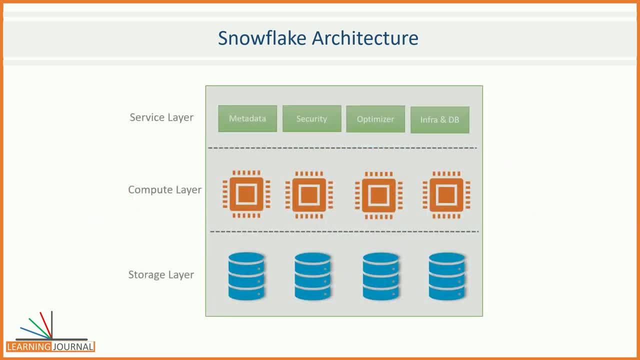 discussion that we had so far. It looks like this: You have databases at the bottom. These are storage only. Then you have warehouses on top. These warehouses are compute only. There is another separate layer which is for managing metadata, security, automatic performance optimizations, transactions and concurrency. 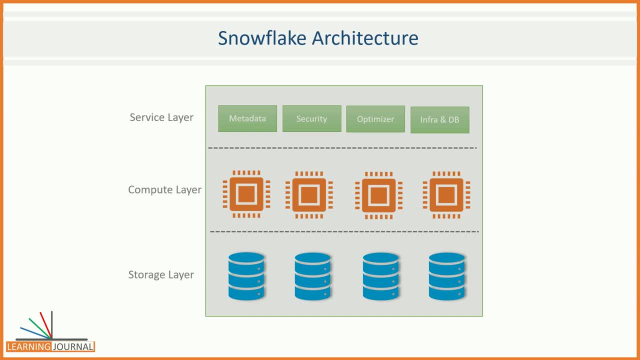 management. This layer is what enables Snowflake to act as a database and comes mostly at a nominal fixed price. Your main cost is associated with the storage and compute requirements. Great Looks, impressive. Not yet. Separation of storage and compute is available with many other. 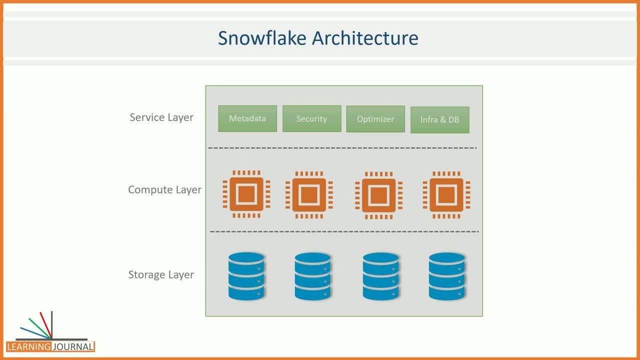 products, Including Amazon EMR and Databricks. You also have a rich enough SQL offered by Spark SQL, So most of those things that I discussed are available with a few other products as well. Snowflake provides a better user experience and makes it simple to implement, But it doesn't make. Snowflake. unique enough yet, Isn't it? Let's deep dive into the database storage layer, And I'm sure you'll be happy with the results you get. So let's dive into the database storage layer, And I'm sure you'll be. 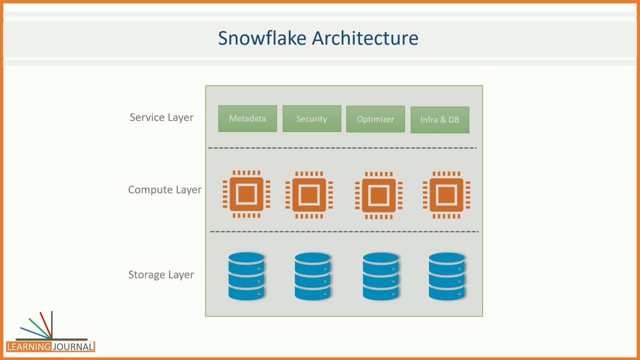 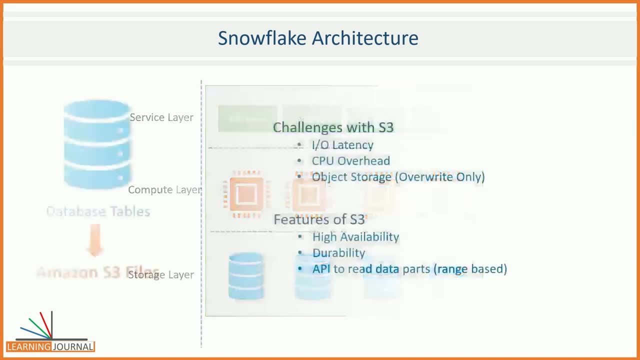 happy with the results you get. So let's dive into the database storage layer And I'm sure you'll be impressed almost immediately. Snowflake decided to use S3 as its storage layer. That was a contrarian decision for database storage, because we all know that S3 comes with a varying performance and put up 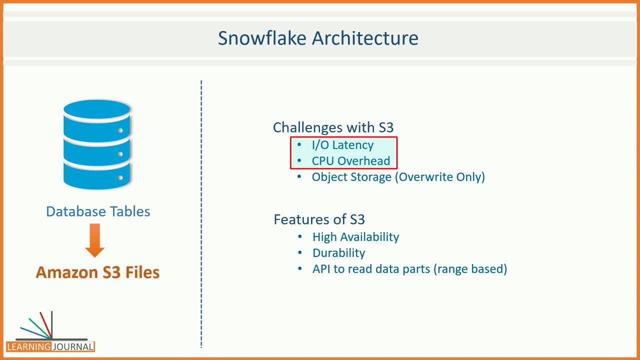 several restrictions. For example, S3 has a much higher latency and CPU overhead compared to the local storage. That is why HDFS on local storage works better than the local storage. So S3 has a much higher latency and CPU overhead compared to the local storage. That is why HDFS on local storage. 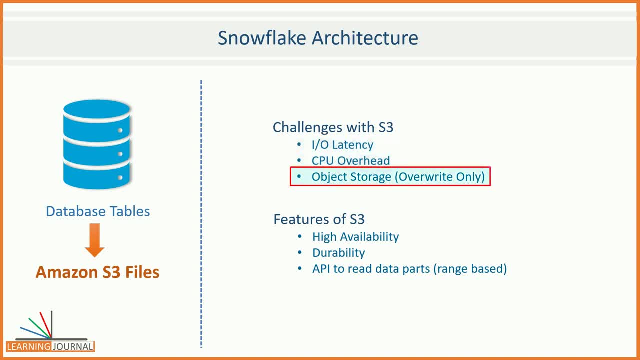 works a lot better than S3.. The second problem: We can only overwrite files in S3. It does not support updating or even appending the same file. These two problems are so critical that they often put a hold on the decision to use S3 as a database storage. I mean you can dump files in there, But using it as a 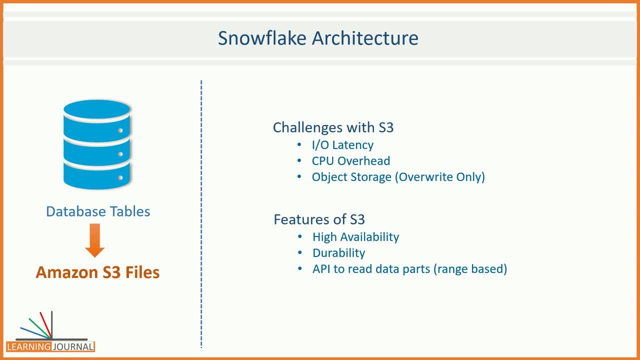 database storage layer would be a no-no talk. So let's dive into the database storage layer, And I'm relying an excellent video by S3TV stem nerf right, Right. However, the Snowflake team found two main technical reasons to use S3.. 3. High availability and scalability. 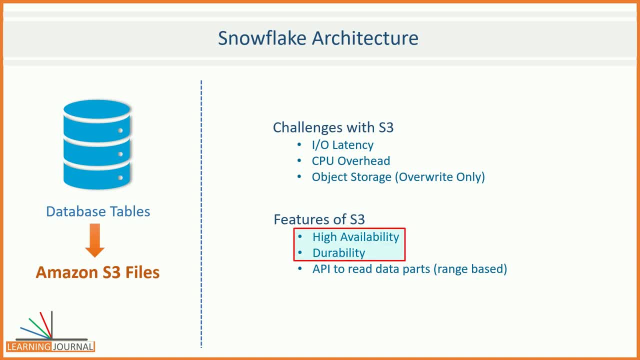 When you change myission data, you already understand these things. You used to need to understand so much more things than having tochl, Kate 3 and ps4 IDE Ai-min Yim S3.. S3 doesn't go down And once saved, you cannot lose your files. 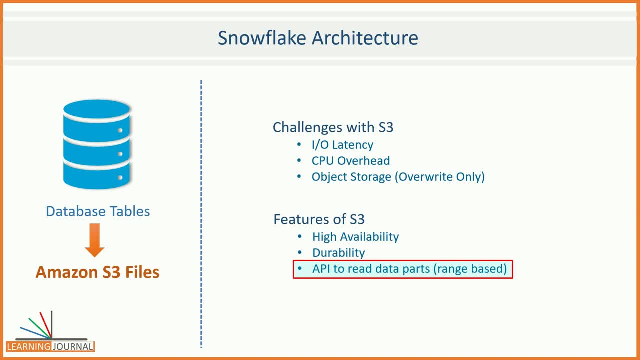 Now the second and most critical reason. S3 APIs allowed them to read a part of the data from an S3 file. What does it mean? Well, the ability to read in parts provides a Macalus functionality for data read in other hard drives that might hide. 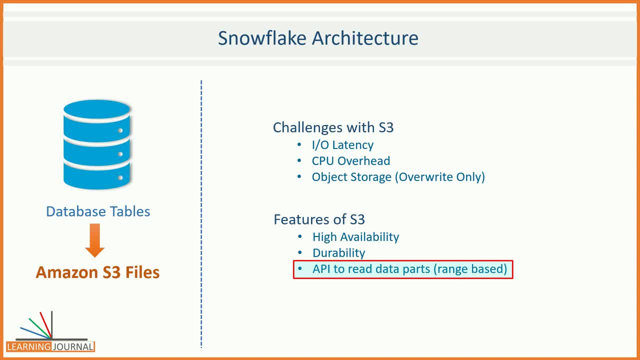 on another list of hard drives without even loading the entire file is a kind of random access capability, isn't it? Not truly, but a kind of right, And that could be a powerful feature if you have something like an index that allows you to read exactly what you want to read and avoid reading unnecessary volumes. 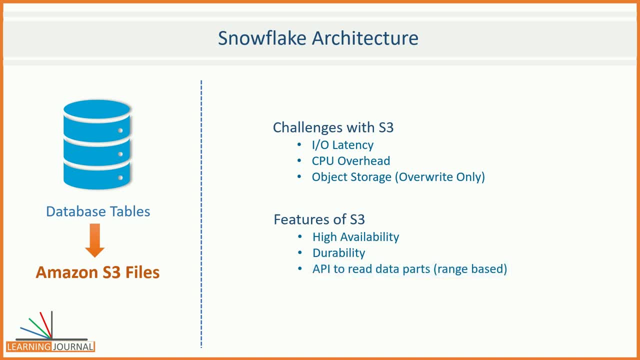 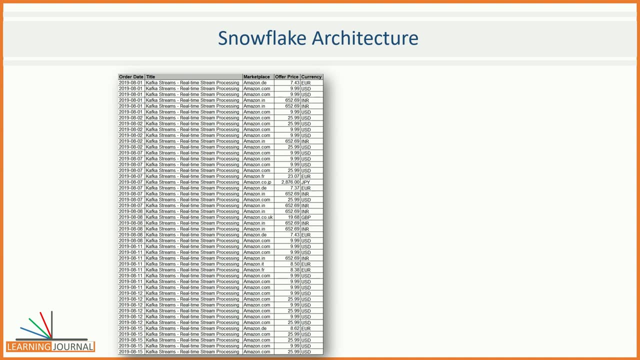 Great. So the next question is how exactly Snowflake leveraged these S3 capabilities. Let's assume that you have a large table. For a simple illustration, consider this table. This one is a relatively small table, but the idea that I'm going to explain is applicable for a super large table as well. 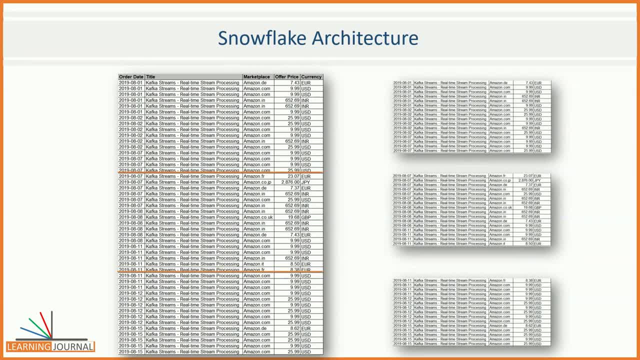 The first thing that Snowflake does is to break the table into multiple smaller partitions- and they call it micropartitions- which is not more than 500 MB in size, So each table partition is between two micro-partitions, which is not more than 500 MB in size. So each table partition is between: 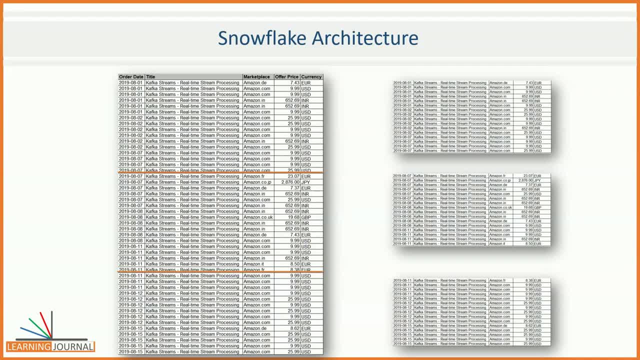 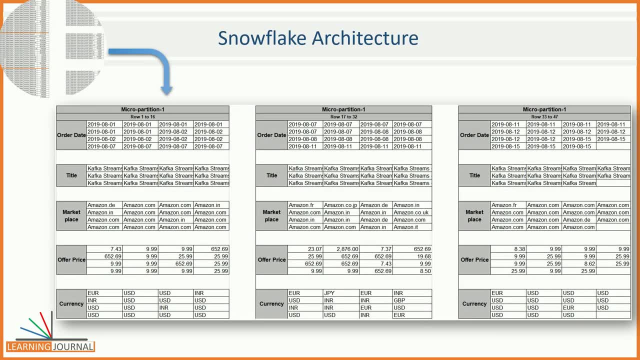 between two micro-partitions which is not more than 500 MB in size. So each table partition is between 50 to 500 MB of uncompressed data. The next thing that they do is to reorganize the data in each partition to make it columnar. 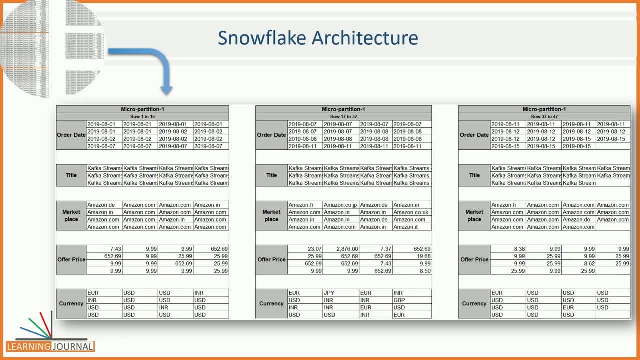 What does it mean? Simple Column values in the partition are stored together. The next step is to compress each column, And that's unique. You are not compressing the entire partition, You are compressing only the column. You are compressing only the column values individually. 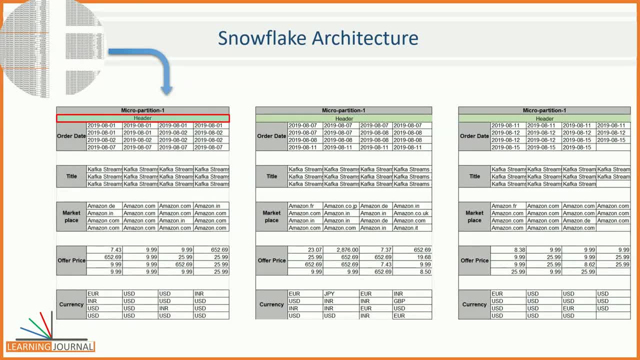 Finally, they add a header to each micropartition. The header contains an offset and length to each column stored within the micropartition. They also store some other metadata information in the header, but the column offsets are the most critical information for us to understand the read pattern. 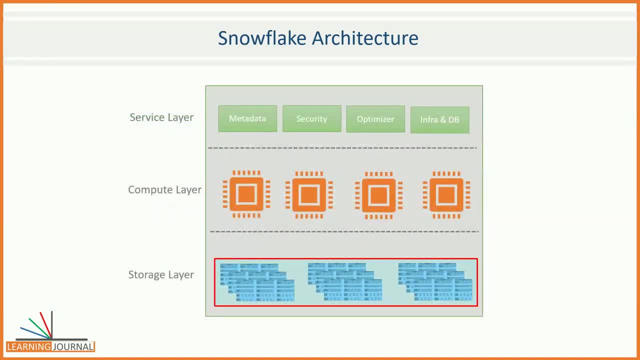 Now these micropartitions are stored in S3 as immutable files And a lot of metadata and statistics about these micropartitions is maintained in the Snowflake metadata layer, And that's why they called the Cloud services layer of the Snowflake as the brain of the 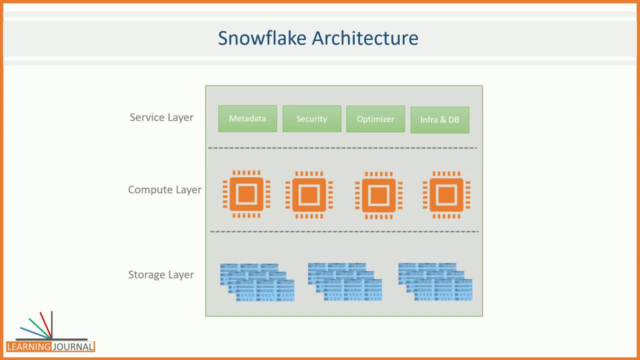 Snowflake. When you fire an SQL query, Snowflake would know which tables and what columns do you want to read? Which micropartition files in S3 belong to the desired studying issue? Moreover, use CSS and JS. Yes, that's 399 unfinished sentences of 2013.. 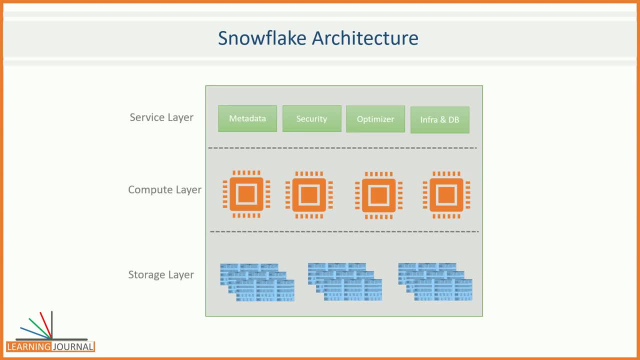 table, So they know which files to read. But instead of reading a complete file, they first read the header and then read only those columns which you wanted to read. And this is possible because S3 APIs allow them to read part of a file based on offset and length. Amazing, isn't it? 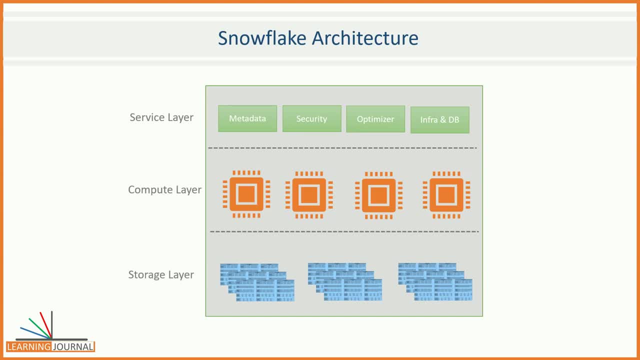 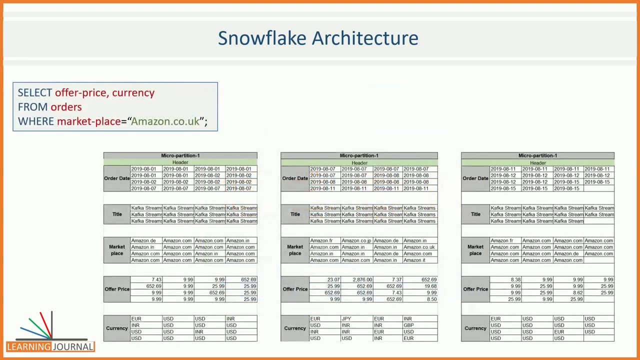 I assume that you are getting a sense of how this storage architecture allows them to optimize their IO operation. Let me elaborate a little. Snowflake stores metadata and statistics about all the data stored in the micropartition, So they know the range of the values and the number of distinct. 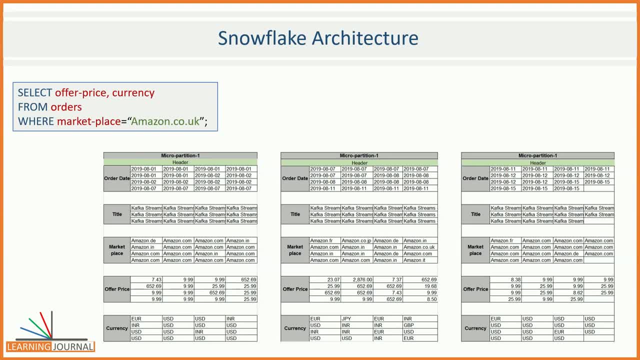 values for each of the columns in the micropartition. So when you apply a filter in a where clause, they know which micropartitions would have the desired data. This allows the first level of partition pruning And targets only those micropartitions where the desired data is stored. In the next step, they first 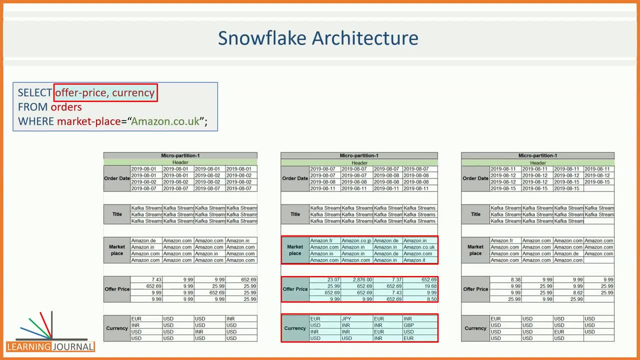 read the micropartition header and then only read the desired columns, And this allows the second level of column pruning and minimize the overall IO for the SQL. In other words, they automatically apply a generic partitioning strategy and columnar storage and take away this headache from the 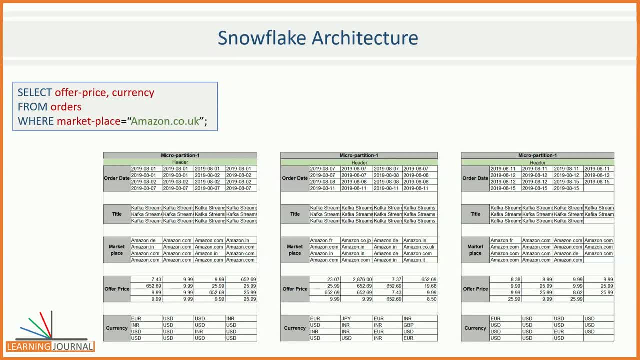 database design. In most of the cases, this generic partitioning works very well due to the tiny size of each micropartition. If you have a time series data and your queries are filtering on a time frame, this partitioning strategy works like a charm In certain other use cases, when you already know your commonly used filtering. 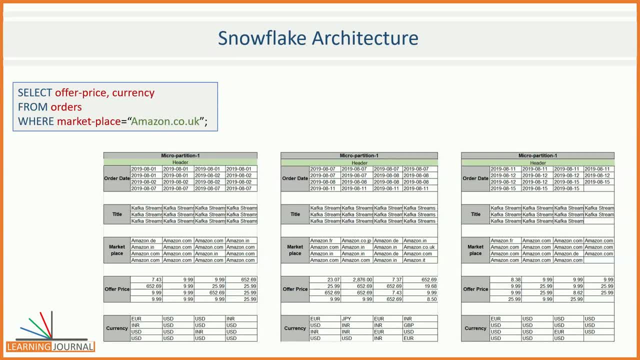 columns. they also give you an option to define table clustering key to increase the degree of partitioning. The notion of clustering key is similar to what we see in Cassandra. That means the data is ordered by the clustering key and stored close to each other. 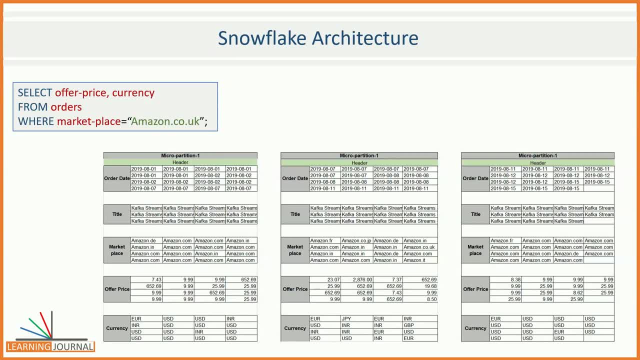 Great. I will cover some more exciting details in part 2 of this video. See you again, Keep learning and keep growing. 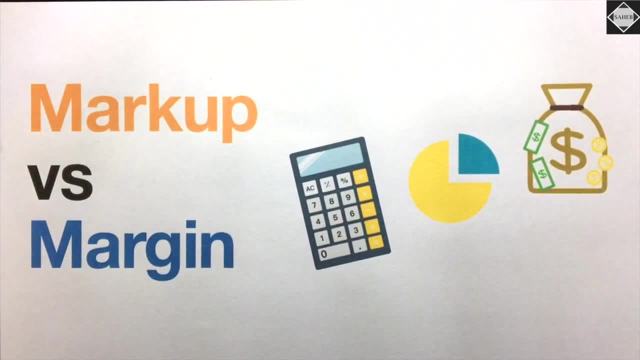 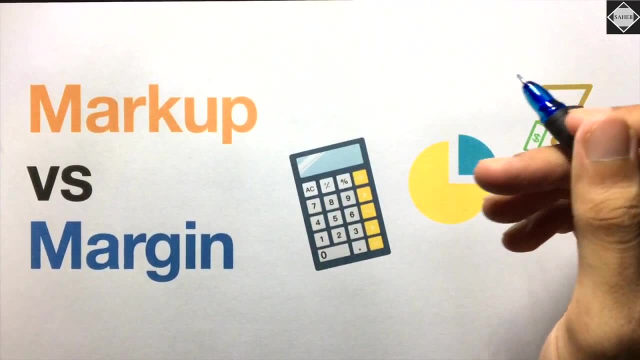 Hi everyone, welcome back to Sahab Academy Today. in this video, we are going to understand the concept of markup and margin, and we'll see how to calculate this with a formula. and then the most important thing is the interpretation You should be able to understand once you know. 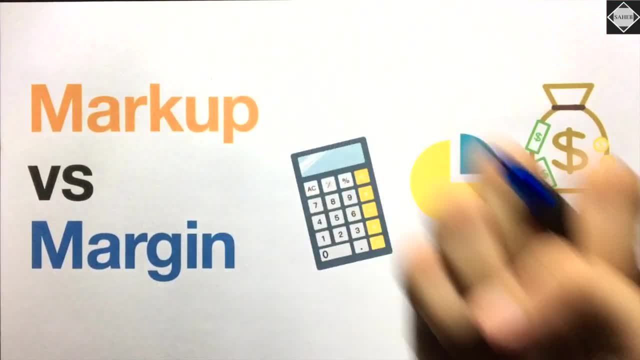 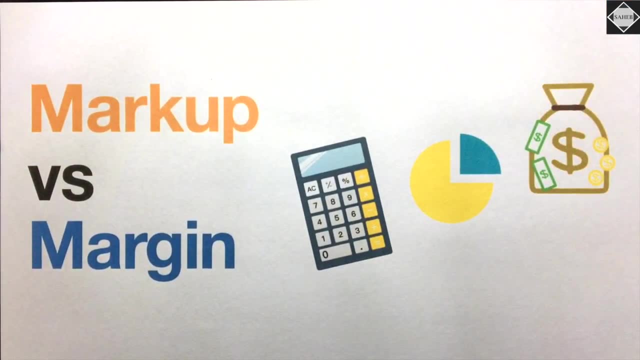 how to calculate the markup and margin. What is the interpretation you can get out of this? That's very important, and we are going to see that with a beautiful example. So let's start the video and let's get into it Now, before getting into the concept of markup and margin. 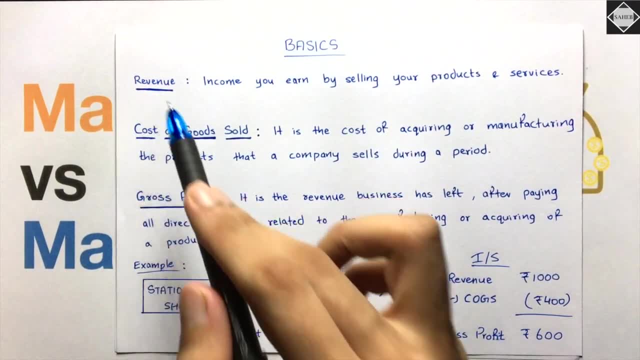 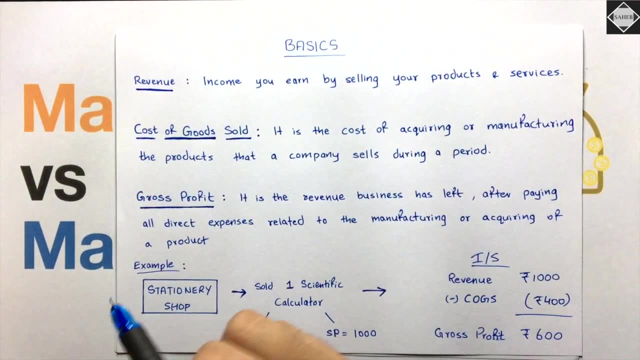 let's just understand these three things of the income statement: Revenue, cost of goods sold and gross profit. It's very simple, See here, revenue is the income you earn by selling your products and services, The main inflow that the company has, the business has. Okay, that's. 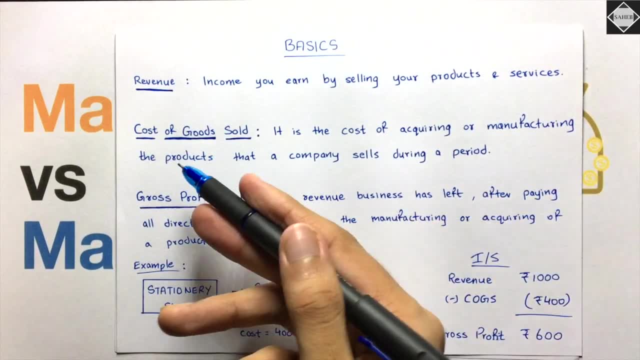 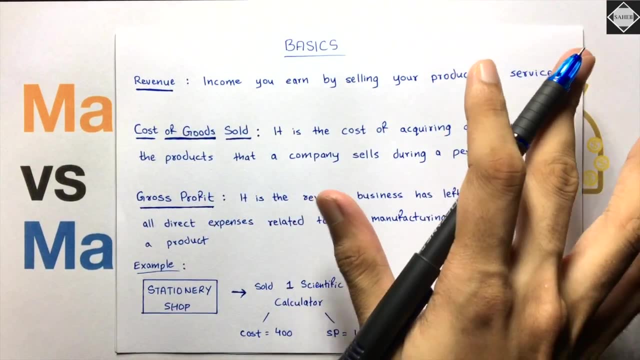 revenue And then what is cost of goods sold. It's really simple. As the name says itself, it is the cost of the item which you have sold. For example, if you have sold five umbrellas costing 100 rupees each, so that 100 is the cost price of the umbrella. Cost of goods sold would. 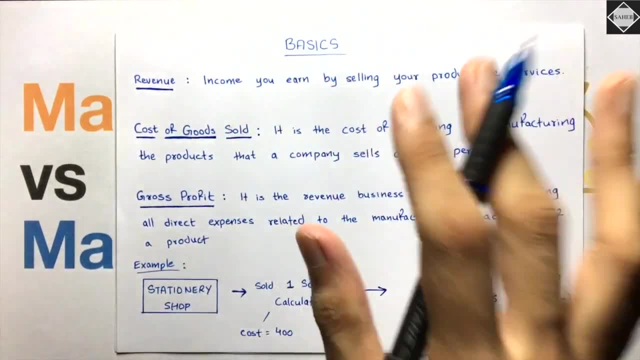 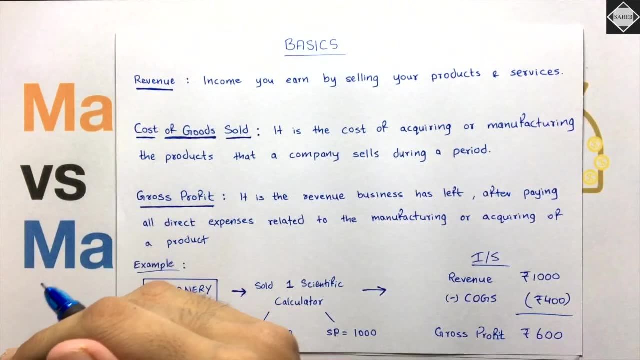 be: how many have you sold? You have sold five, So five into 100, that's 500.. 500 rupees would be your cost of goods sold And in your stock, in your- what do you say- store, you have so many.